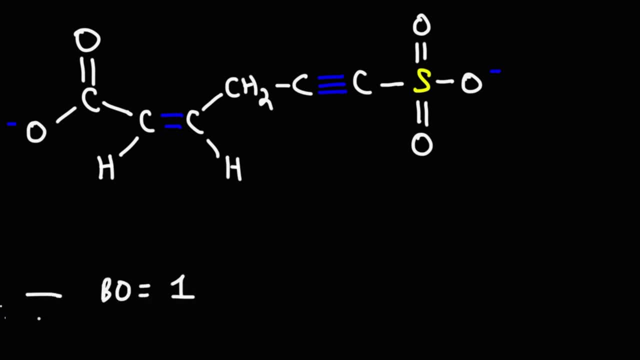 single bond, the bond order is 1.. For a double bond, the bond order is 2.. And for a triple bond, the bond order is 3.. Now for bonds that are involved in resonance, you can have fractional bond orders. So for the C-H bond, that's simply a single bond, so that's going to have a bond. 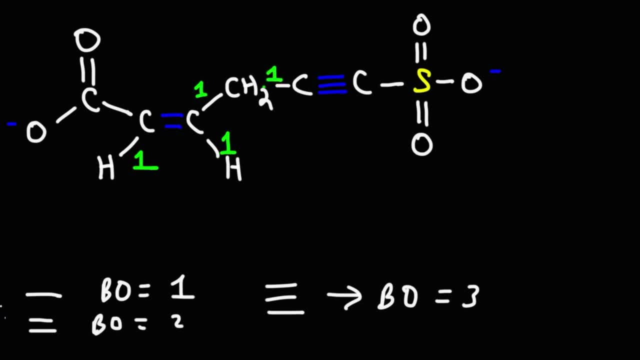 order of 1.. Every single bond that we see here that doesn't participate in resonance has a bond order of 1.. The double bond has a bond order of 2.. The triple bond has a bond order of 1.. The triple bond has a bond order of 3.. 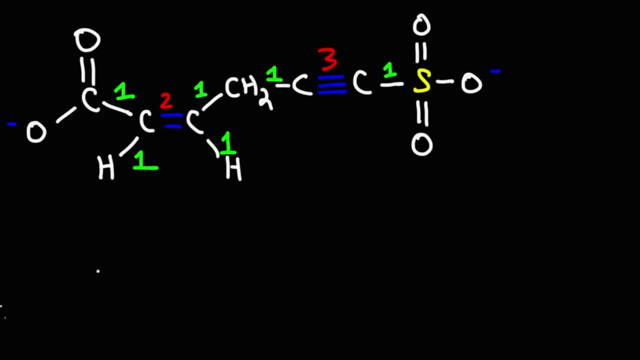 Now let's focus on this group right here. I'm going to redraw it like this And let's show the lone pairs. So we have two lone pairs on the carbonyl oxygen, three lone pairs on the other one. Now, if there were no resonance structures, 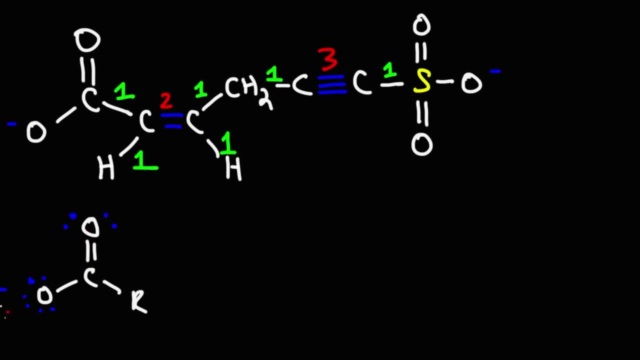 you'd assume that this bond would be a bond. But if there were no resonance structures, this would have a bond order of 2.. But because we can draw a resonance structure, the bond order is going to be different. If we take a lone pair, we can use it to form a pi bond and we can break this pi bond. 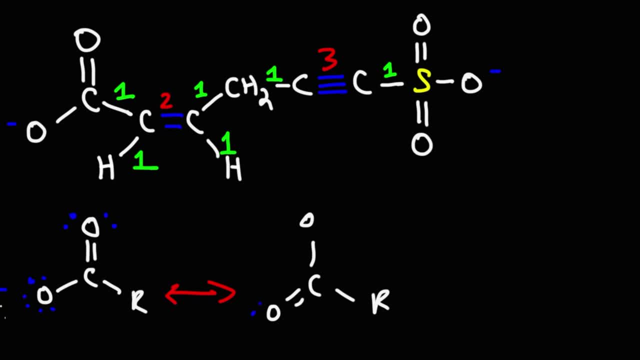 put in two electrons on that oxygen. So this oxygen will now have 2, the other one will have 3 and the negative charge. So now, looking at this particular bond, would you still say it has a bond order of 2? Because here it looks like it has a bond order of 1.. It turns out that the actual answer is going: 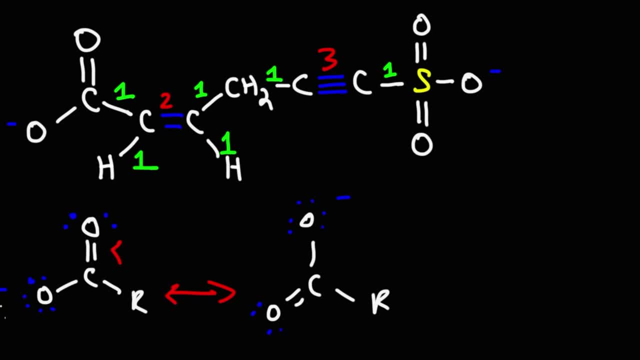 to be an average of those two numbers, It's 1.5.. So the way you would calculate bond order is you would look at the number of bonds of the atoms that participate in resonance. So that would be three bonds here, And you would divide those three bonds which. 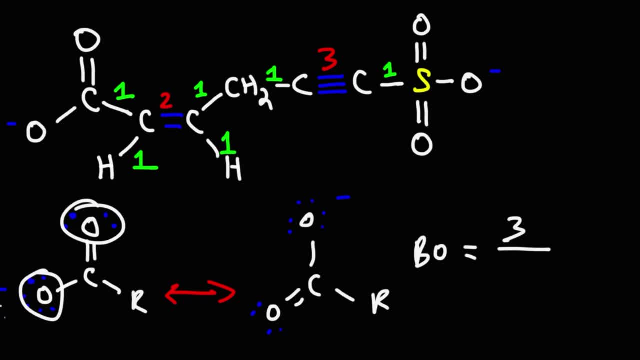 are basically part of those two atoms. So those three bonds are connected to those two atoms, not including the central atom. So you could think of it as the three bonds being shared across two atoms. So you get a bond order of 1.5.. And it makes sense. Here it looks like it's 2.. Here